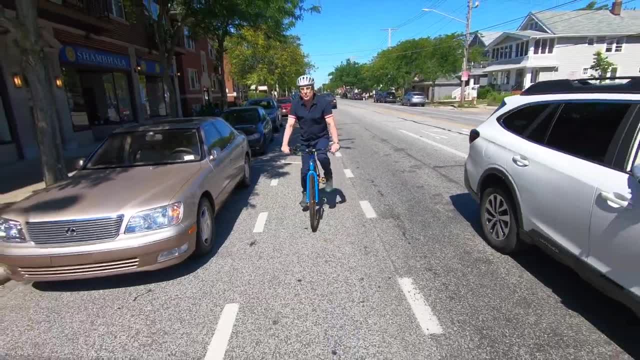 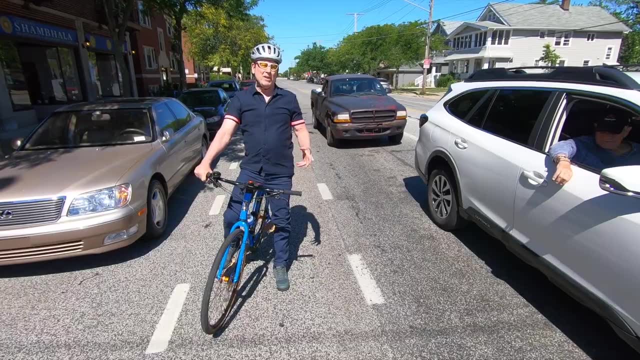 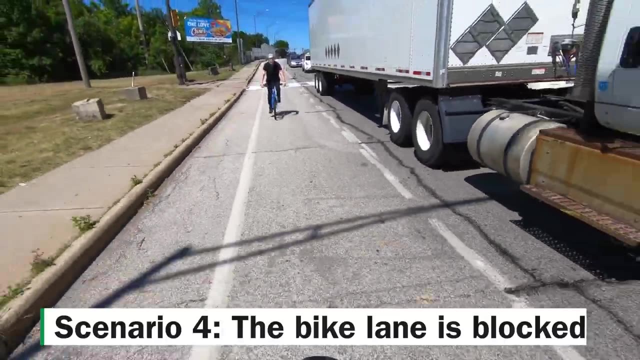 area and avoid the door zone or you might get doored. but you have to also be careful because people might not park absolutely correctly and if they park incorrectly the door zone could be even further out. things get a little funky here. there is a truck blocking the bike lane. 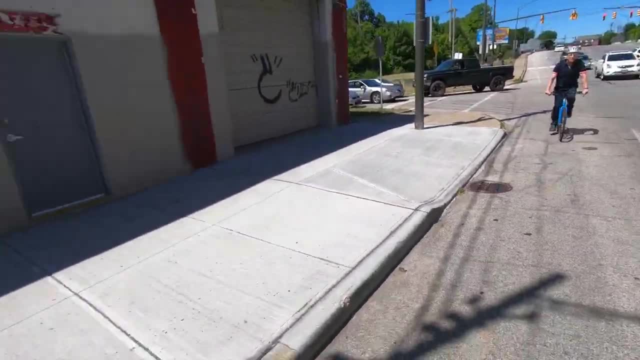 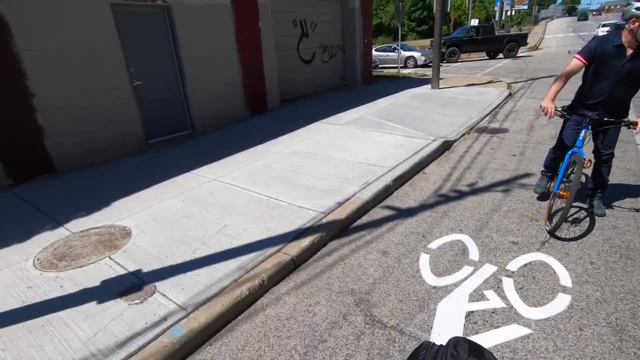 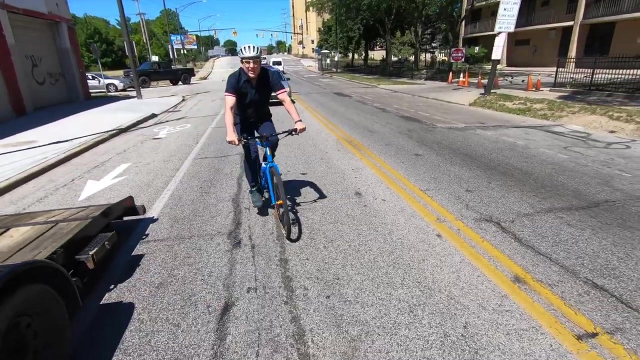 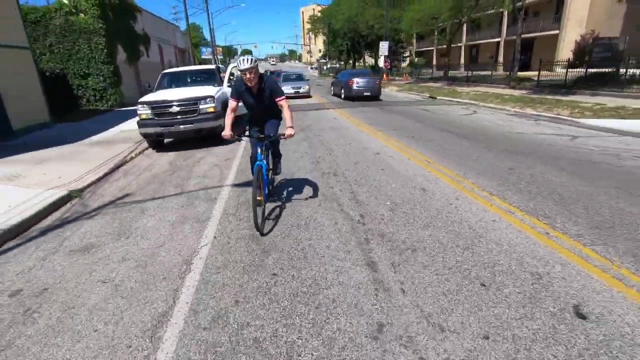 with its flashes on. it's illegal to block the bike lane unless you're stopping for a brief moment, so we have to get around pointing to the car behind us. that's what we're doing and we're going to roll back into the bike lane, but there's another parked car in the bike lane, so we're going to stay to the 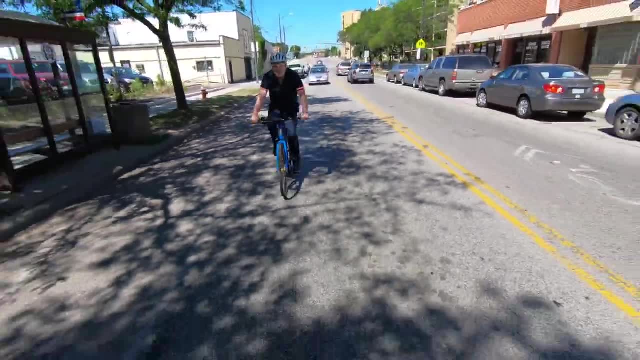 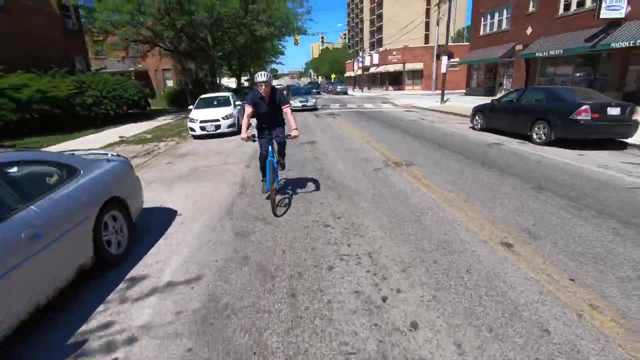 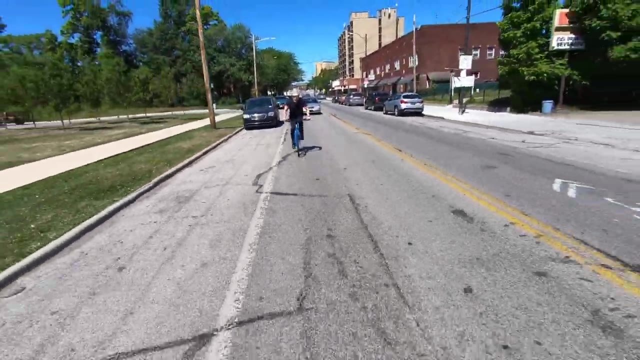 left. you have every right to ride in this lane too, just like any other vehicle. you're supposed to ride to the right, unless you can take the whole lane because it's too narrow to safely pass. but to the right doesn't mean to the right edge. to the right just means where. 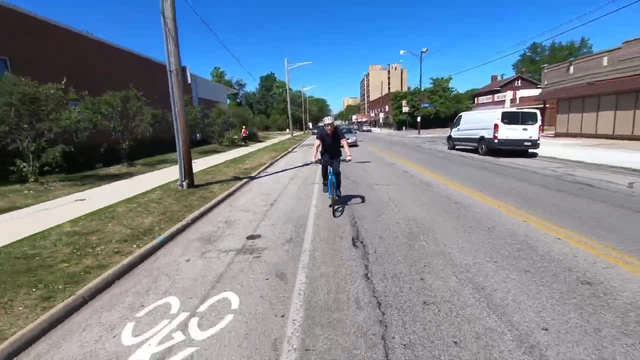 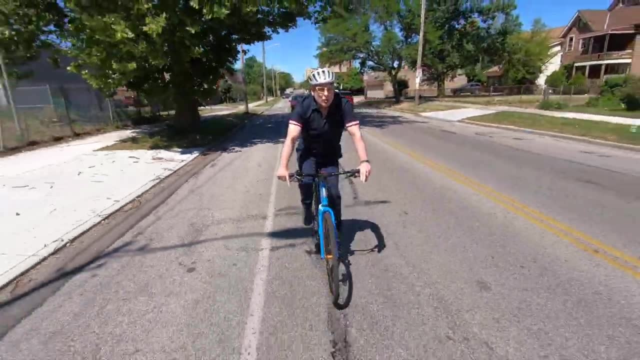 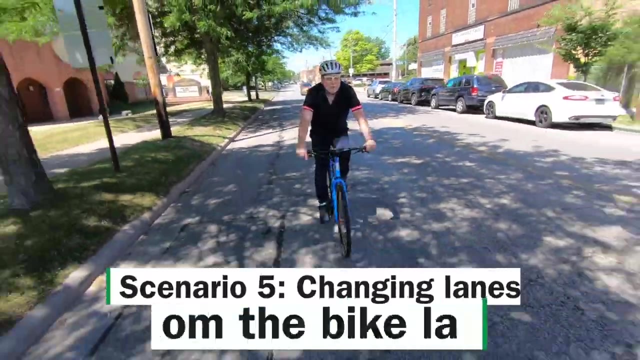 it's safe. so if there's a pothole or debris or someone in the right lane blocking you, making it unsafe, you don't have to ride to the right edge by any means. it's to the right as practicable. okay, we got a right turning lane with a. 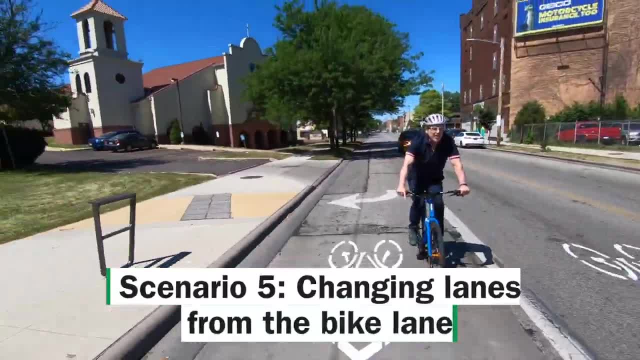 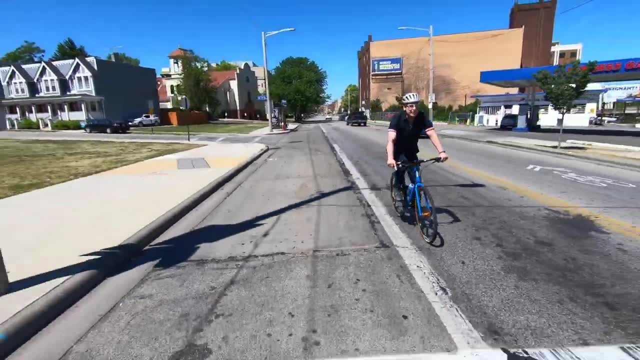 Shero and a left lane. we're going to move into the left lane and we're going to take that left turn. the right turn is the left lane because we're going straight. I'm going to point to that. oh, thank you, car. gonna point to the car. 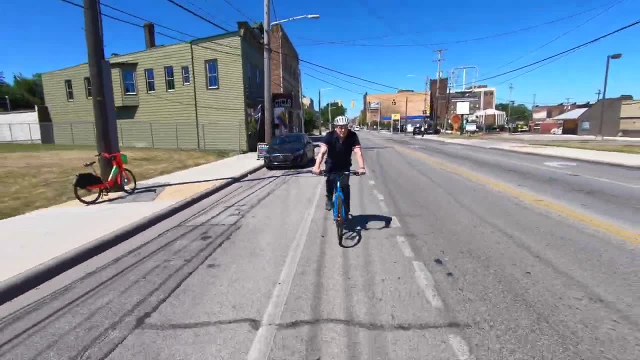 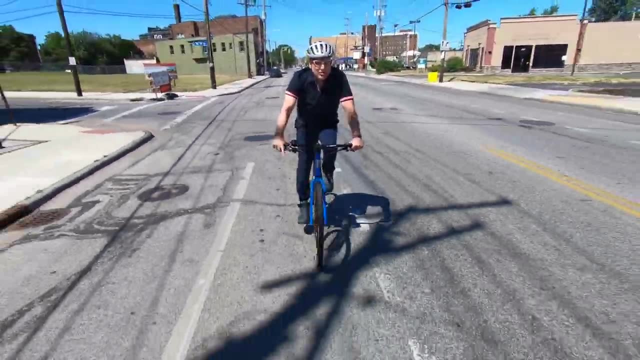 because now I have the right away here. it's a real danger when you go left that the cars don't appreciate that you have to do that and sometimes won't let you, so always look with drivers, give us some room and allow us to move left, because 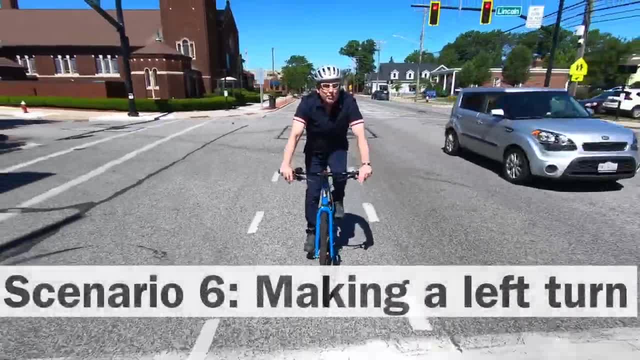 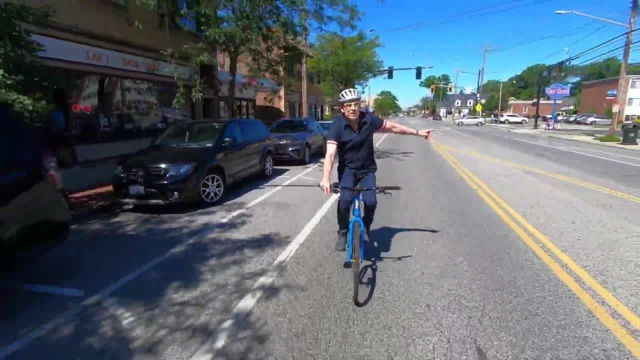 that's how we sometimes have to go, especially to make a left turn. okay, I'm law office, I know I have to get to the left. I look to make sure it's clear. Give it a little point. I see it up there. I see the turning lane. I'm going to merge into the. 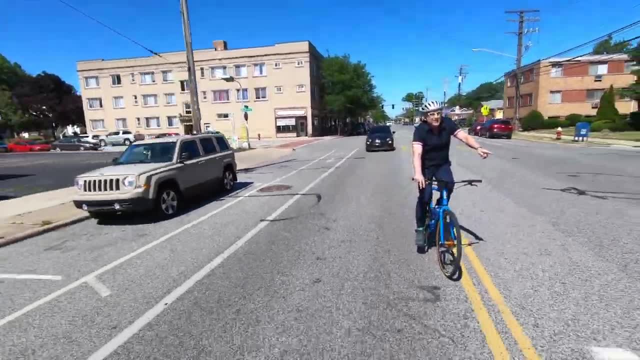 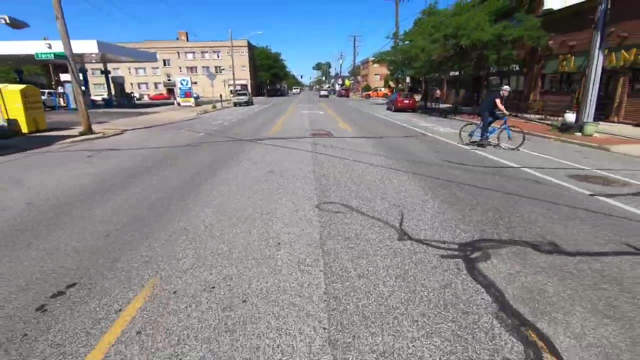 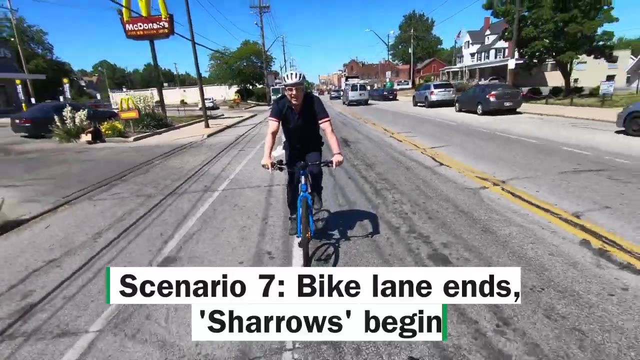 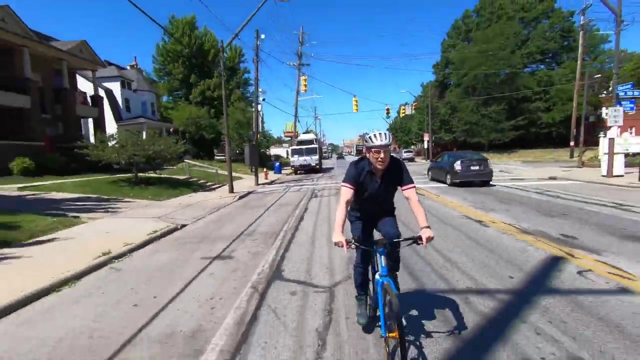 turning lane And I'm going to take the left here. It gets interesting here because the bike lane ends and sharrows begin And the sharrows and a sign says cyclist may take the whole lane. So right about here you'll see the bike. 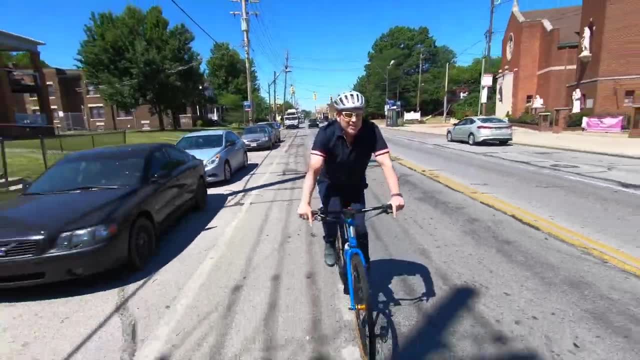 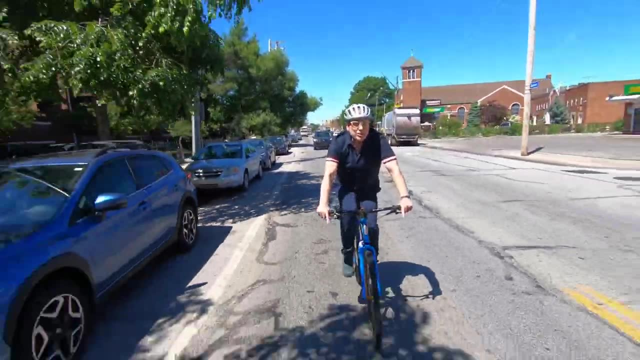 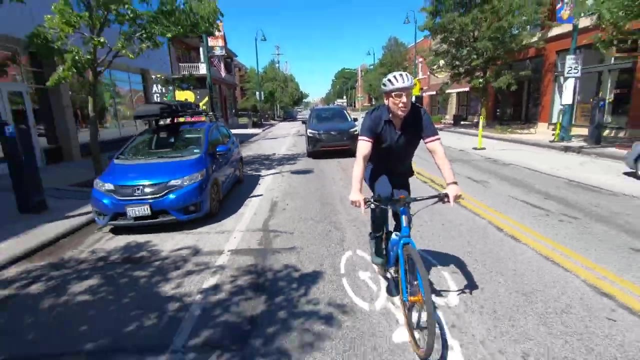 lane end And at this point you can take the whole lane, And you want to do that because the car behind you won't pass you and possibly hit you because there's not enough room, Because the bike lane ended. So here we are taking the whole lane, heading into that green. 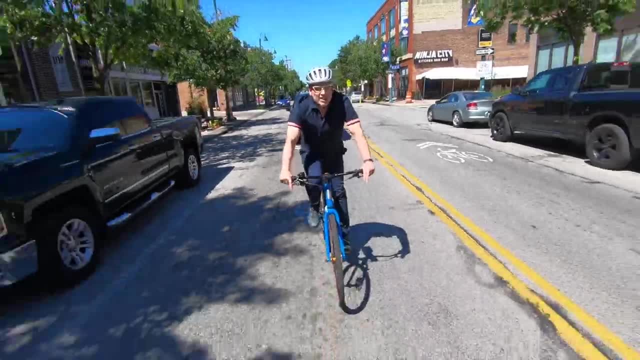 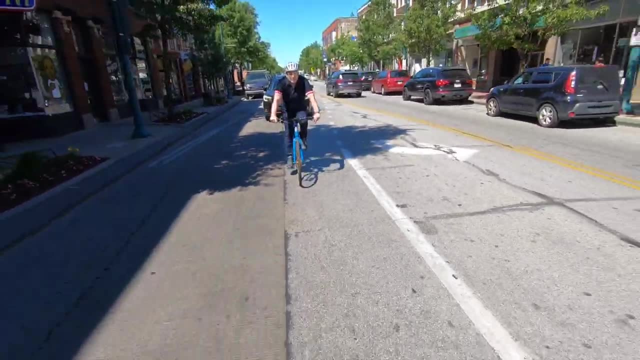 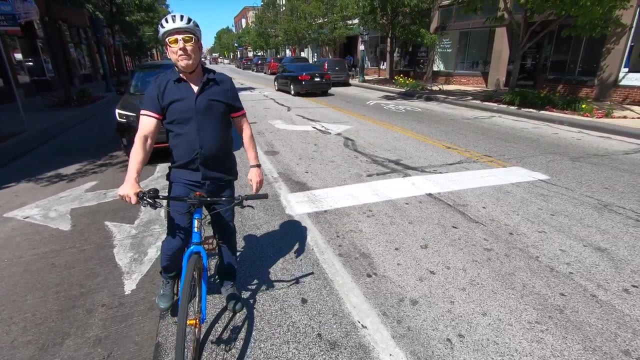 light, which is now red. So when we go through this light on green, I'm going to take the whole lane. I'm going to be right in the middle of the lane so everybody sees me oncoming left, turning cars, Cars passing behind me before I move back into the bike lane. 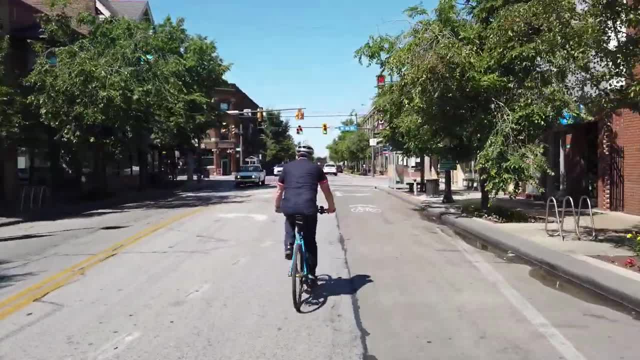 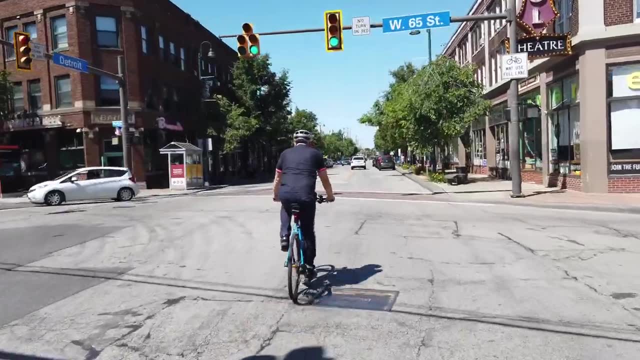 We're heading into the intersection and I'm taking the right lane. I'm going to take the whole lane because I want that left turning car to see me: Nice and safe, Highly visible. Here I am through the intersection. There's another sharrow telling the cars behind me. 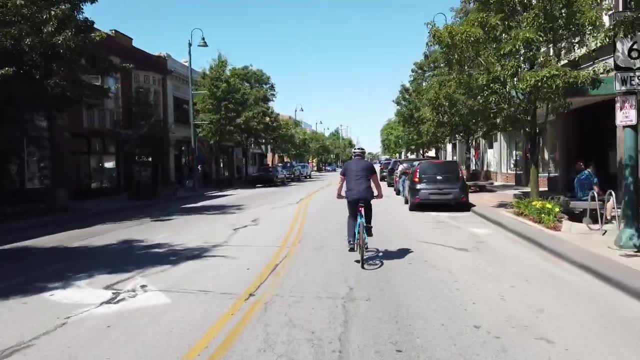 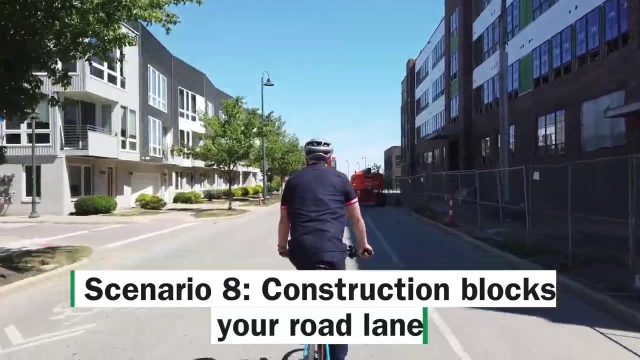 I can take the whole lane, Which I am doing, Got a little construction in front of me here. I no longer have the right of way. If I'm going to go left of center, the car has the right of way. I'm going to let that car pass And I'm going to cross over on the double. 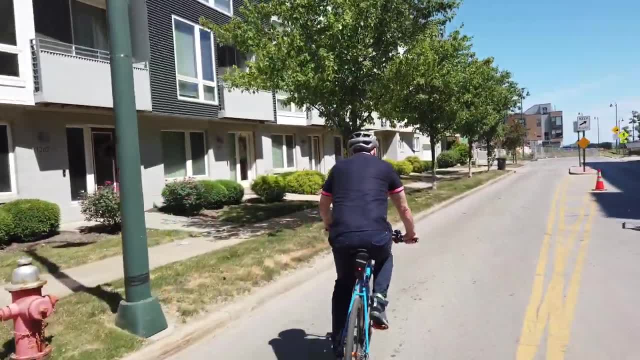 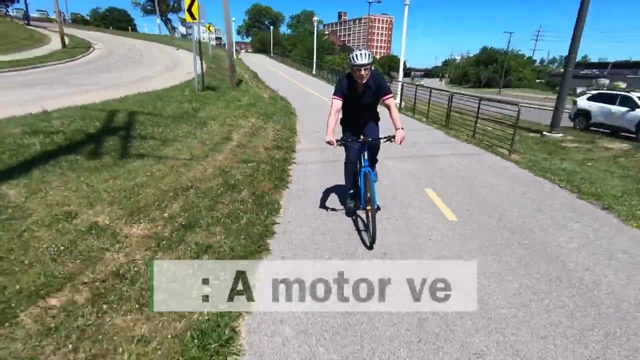 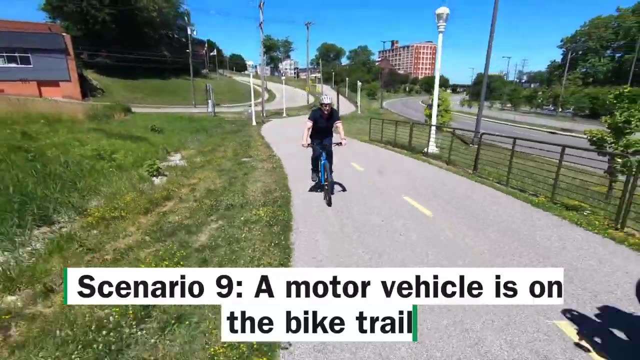 yellow. By the way, a car can pass us on the double yellow as long as the car is not exceeding the speed limit. Here comes a cyclist barreling down. If I was stuck in the left lane, like right now, that's not even a cyclist, That's a motor vehicle, which absolutely shouldn't. 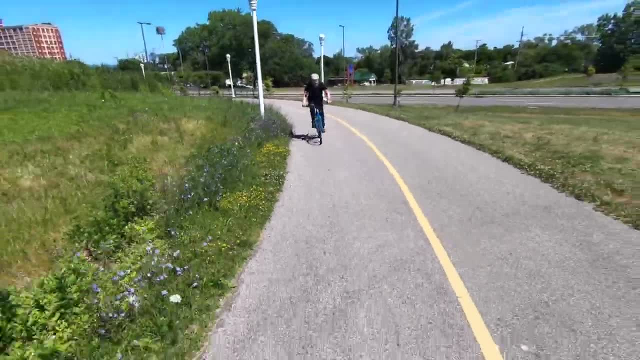 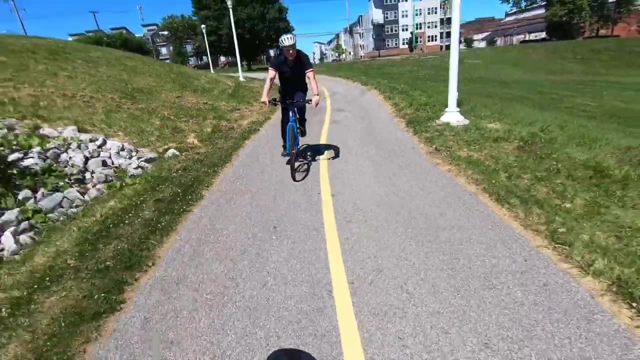 be on this trail, But that's what you get. Be ready for anything. You see the yellow line. Don't go left of it. Even if you're right in the middle of the lane, you're still driving. Even if you're riding two abreast, stay to the right and let the oncoming cyclist